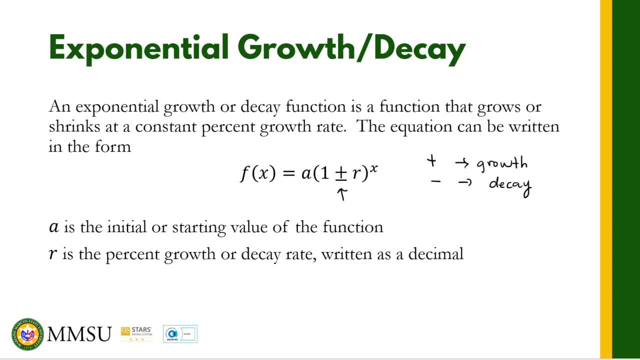 this whole thing. the 1 plus or minus r is greater than 1.. That means we have used plus there, 1 plus the rate. We have an exponential growth. Okay, so let us take a look at the following equations and let us determine if we have an exponential growth or exponential. 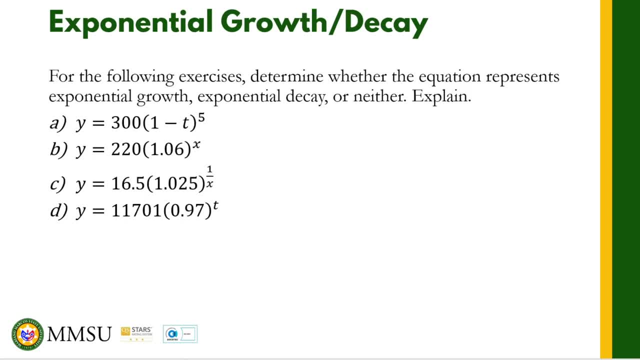 decay, The first one we have. y is equal to 300 times 1 minus t raised to five. So the instruction here is to determine whether the equation represents exponential growth, exponential decay or neither, and please explain. So for letter a, remember the definition of the definition. 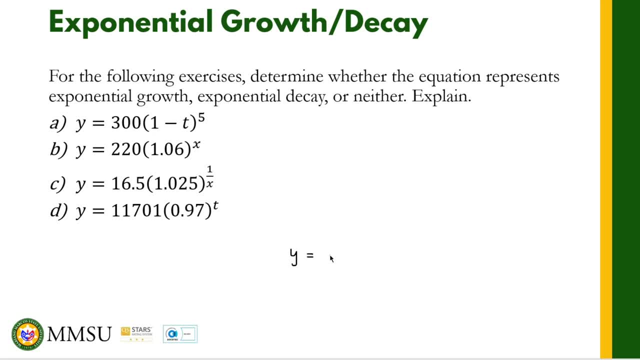 of exponential function we should have: y is equal to ab raised to x. Our independent variable should be in the exponent. In this case our independent variable isn't the base, So our exponent is a real number and not a variable. This means our answer is neither. 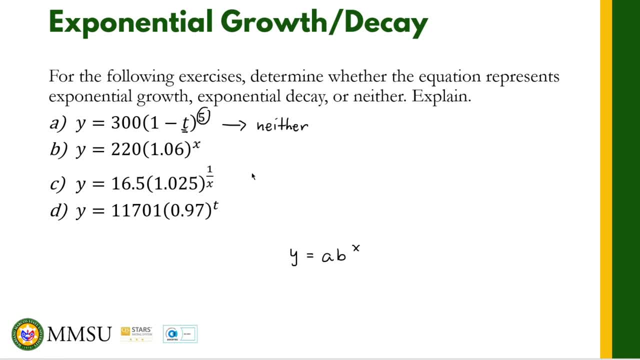 This is not an exponential growth, neither an exponential decay. This is actually a power function, not an exponential function. Okay, for letter B we have: Y is equal to 220 times 1.06 raised to X. You see, the independent variable is on the exponent, so that's okay. 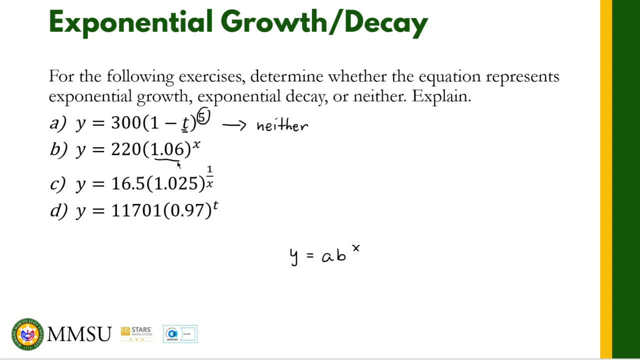 Let us take a look at the base. This is 1.06, that is greater than 1.. That means we have an exponential growth. Okay, so we have an exponential growth. For letter C we have: Y is equal to 220 times 1.06 raised to X. 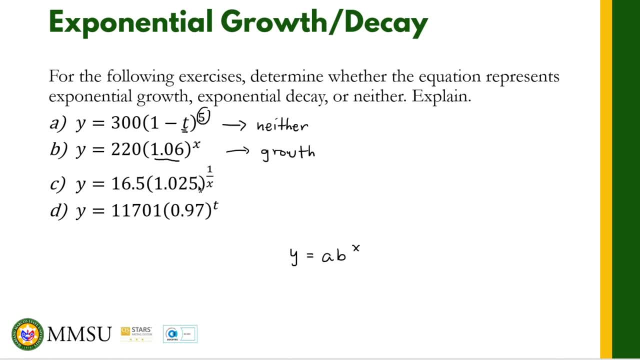 Y is equal to 16.5 times 1.025 raised to 1 over X. As you can see, here our exponent is in fraction form. Okay, but our independent variable is on the denominator of the exponent. This means that this is not an exponential function. 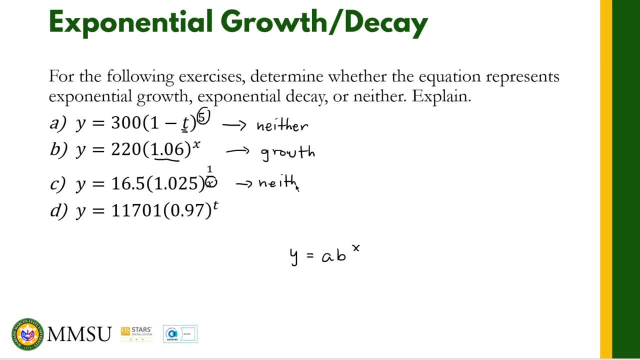 Okay, so we have neither. This is not an exponential function because the variable is on the denominator. Okay, for letter D we have. Y is equal to 11701 times 0.97.. The base is 0.97 raised to T.